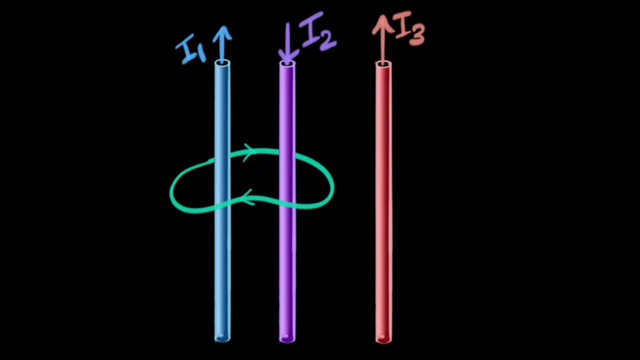 And now comes the important part. He says at every point, and I'll write this at every point: find the dot, product of the magnetic field, and a tiny length DL vector. Okay, what does that mean? So here's what Ampere is saying At every point in space, the three. 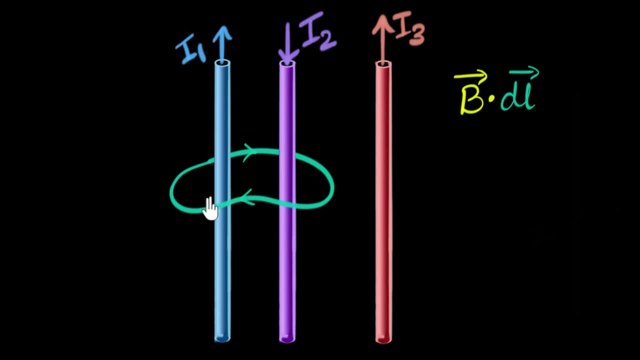 currents are together producing a magnetic field, right? We know that current produces magnetic field, So maybe at this point I'm just drawing random directions. Now, maybe the magnetic field is this way. Maybe there's a point over here where the magnetic field is, I don't know. 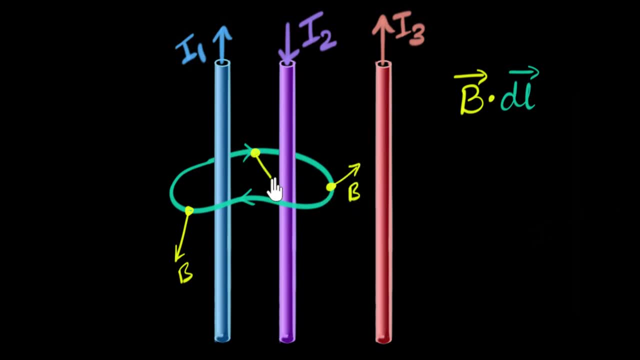 maybe this way, And maybe there's a point over here where the magnetic field is this way. Now, what Ampere says is that, as I'm walking at every point, take a tiny step length, which is DL, and you'll have a direction of this, you know. 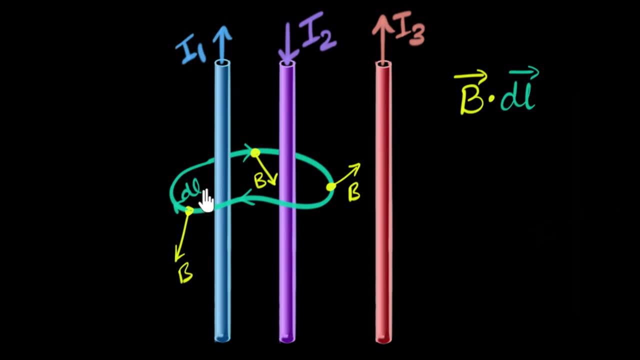 tangential to this path. So over here, DL would be this way. Over here, DL would be this way, And over here, because I'm walking like this, DL would be this way. You can imagine DL to be a very tiny step, like a nanometer or something. It's an infinitesimally small step, And take a dot product. 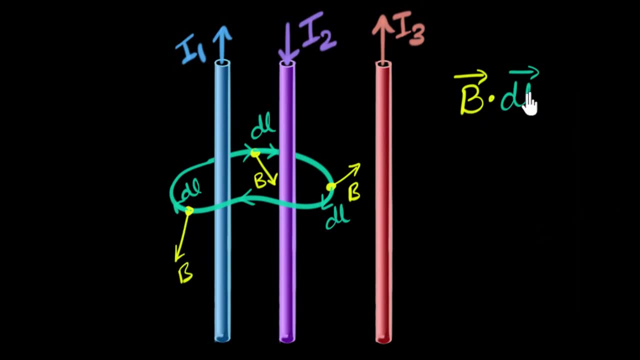 of them, scalar product of them. So BDL, cos, theta, you might know how to take the dot product by now And do that everywhere. And he asks us to then take a summation of that. So add all of that up over the entire loop And since we're dealing with infinitesimals, we're dealing with calculus. 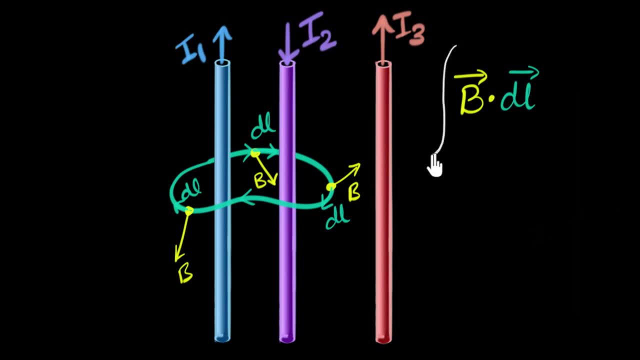 addition in calculus, summation in calculus, is what we call integral, And so this is what Ampere wants us to do in that closed loop. Take the integral of B, dot, DL everywhere. Now Ampere is warning us- not warning, sorry- reminding us that this will only work for closed loops. 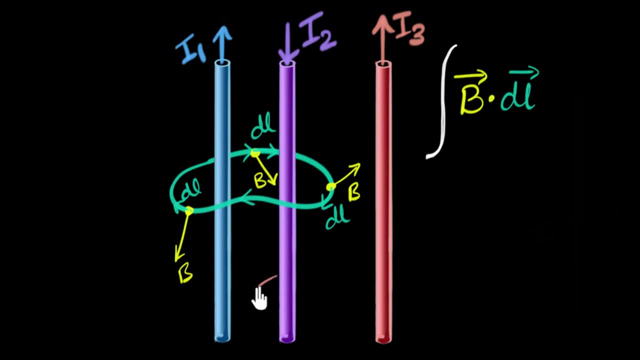 For example, if I had chosen, say, a loop which looked like this, then it will not work. Ampere says: don't take this. Even here I would take, I can take B dot DL, right. But Ampere says no, no, no. 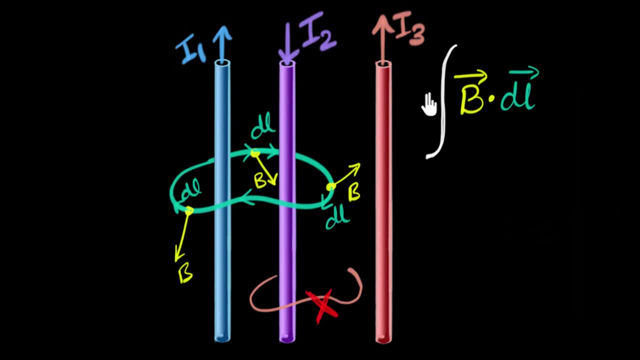 only for closed loops. And so to remind us he's going to put a circle over here. Oops, Let's use the same color Circle over here And it says closed loop. All right, All right, What happens if I do that? Ampere asks me: Mahesh, what do you think will happen if you took this? 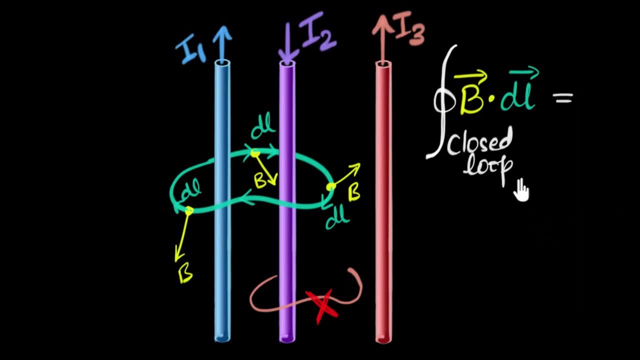 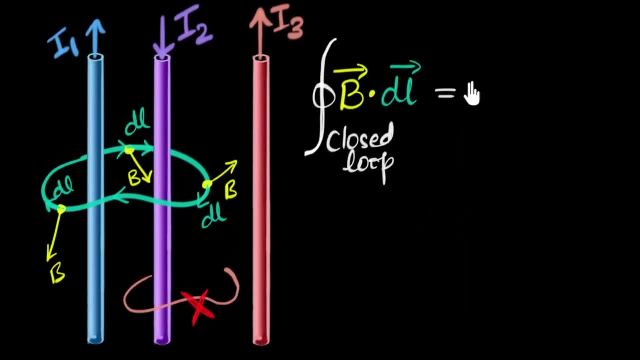 integral over the closed loop And I say I have no idea. You tell us Ampere, This is where Ampere smiles and laughs and says, ha, the answer is going to be: and this is the, this is the Ampere. 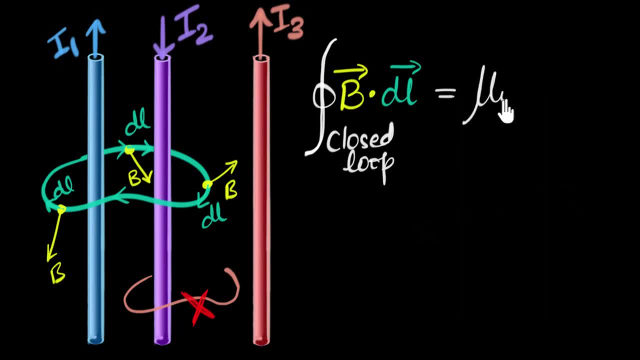 circuit of law? The answer is going to be always mu naught times. I n closed. And this, my dear friends, is what we call the Ampere circuit of law. It's called circuit of law because it has a path involved, And paths are usually called circuits. You may have 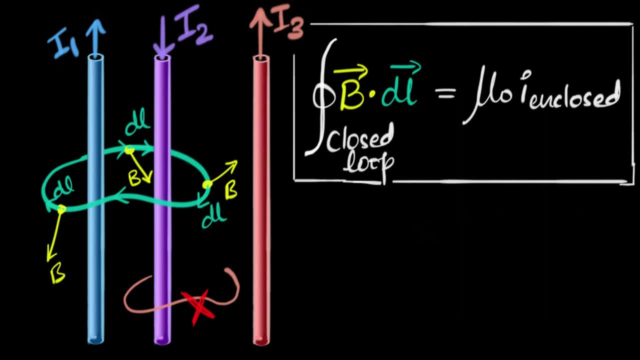 uh, heard of that- in racetracks. Racetracks are also called circuits. Now, before we continue, I'm sure a lot of questions are brewing up in your mind, Like: why do we need this law? Well, as we will see in future videos, we can use this to figure out the strength of the magnetic. 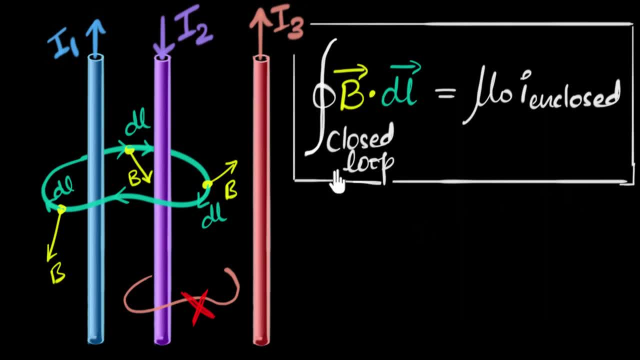 fields in certain symmetric situations. We'll do that in the future videos. Okay, But for now, let's concentrate on the right-hand side and ask ourselves: what does this n closed current mean? Well, let's ask Ampere, Ampere, what is this n closed current? Well, 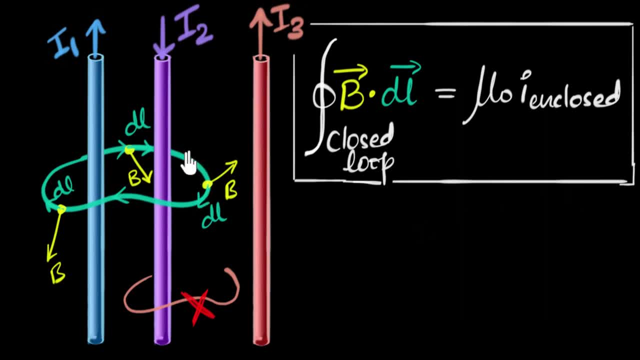 one way to think about this is basically how much current is n closed, the total current n closed by the loop. But Ampere is a little bit more specific. Ampere says: look to figure this out. first step you have to do is attach a surface to this loop, And I don't understand that. I ask: 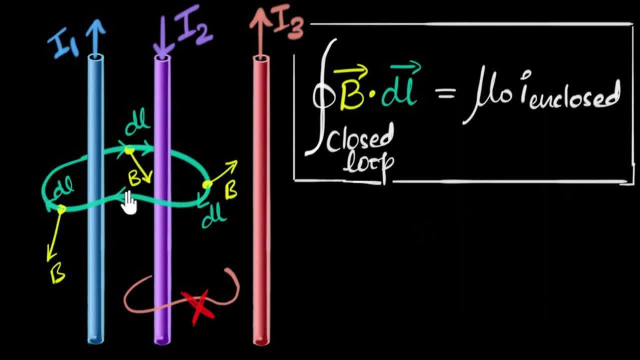 Ampere, what do you mean? So Ampere says: okay, imagine this. Imagine you took this and dipped in a soap solution. What would happen? There'll be some soap film attached over here. right Here you go. Let's imagine that's the soap solution. 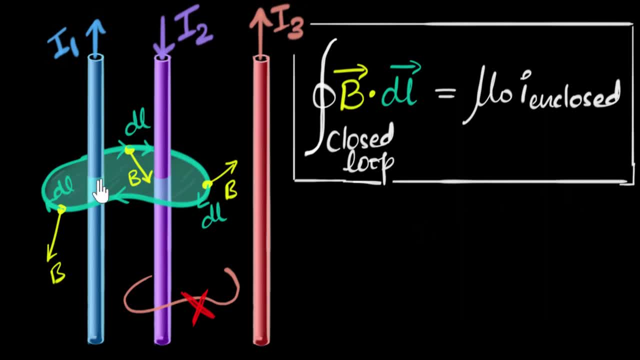 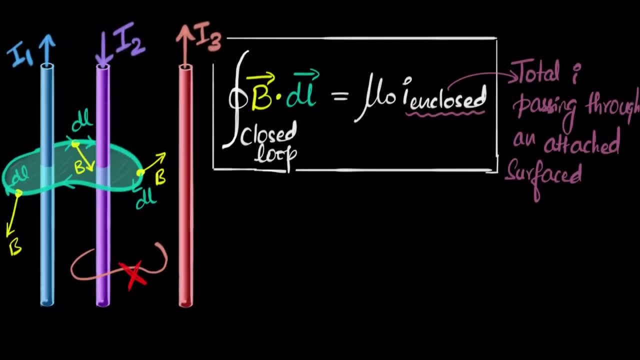 Now Ampere says n closed current is the current that punches through this surface. Whatever is punching to that surface is the n closed current. So the n closed current is basically the total current that is passing through an attached surface to the loop. The attached surface is: 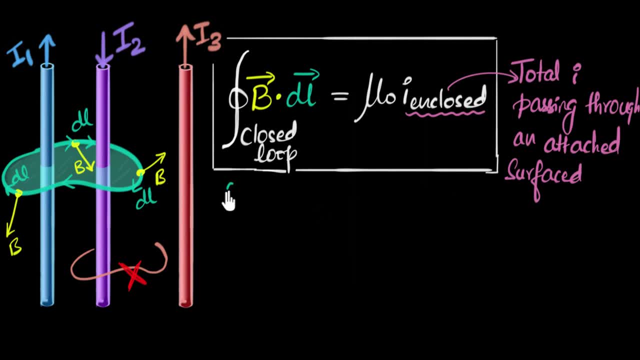 our soap solution. So, in our example, what would be the value of b dot dl according to Ampere's law? Well, that's going to be mu naught times. what is i n closed? Only i. when i2 are passing through the attached surface, They are the only ones n closed. i3 is not, So i3 will. 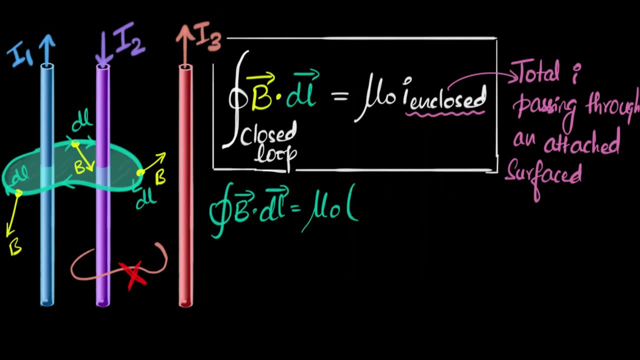 not be in the picture. So the total will be: total will be i1 plus i2.. But the moment I write that I feel uncomfortable because I know that one current is going up, another current is going down. So one must be positive and one must be negative. right, Ampere says yes, one must be. 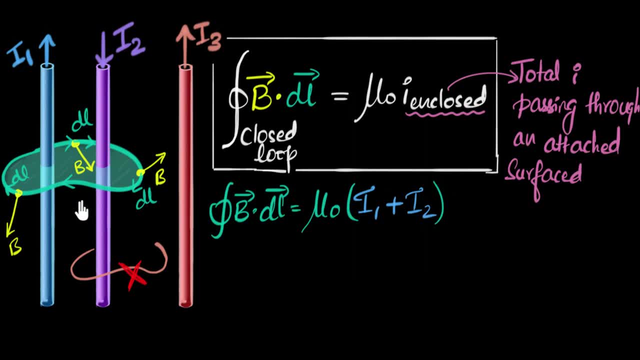 positive, one must be negative. but how do I figure out which one is positive and which one is negative? What do I do? So Ampere says we use the same thing that we've used so far in magnetism: right hand rule. 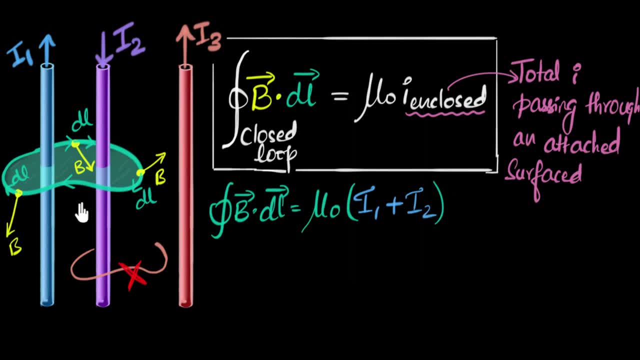 He says: take your right hand and curl it in such a way that the curved fingers are in the direction of your travel And then the thumb represents the positive direction. So in our example, since I'm traveling this way, if I take my right hand, 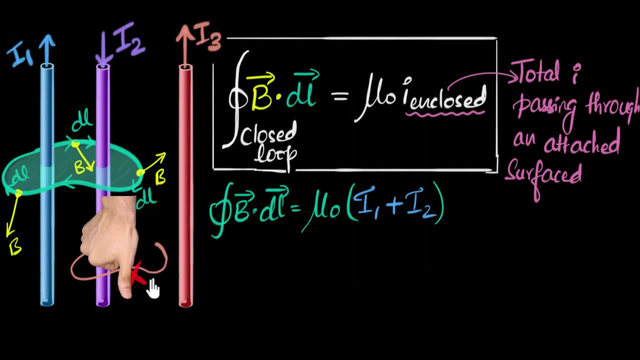 and if I curl my fingers in that direction, my thumb will point downwards, And so this means, according to my right hand thumb rule, downward direction is positive for this loop. So I2 would be positive, I1 would be negative. So this is now the correct application. 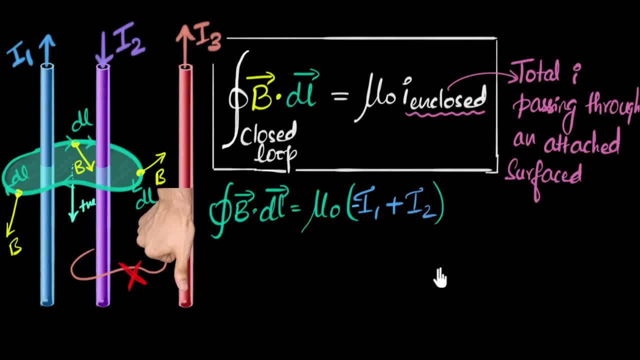 of Ampere's law for this case. Why don't you quickly try one? So let's say, let's take another loop which is over here. We're gonna take a rectangular loop because shape doesn't matter. So let's say we take a rectangular loop. 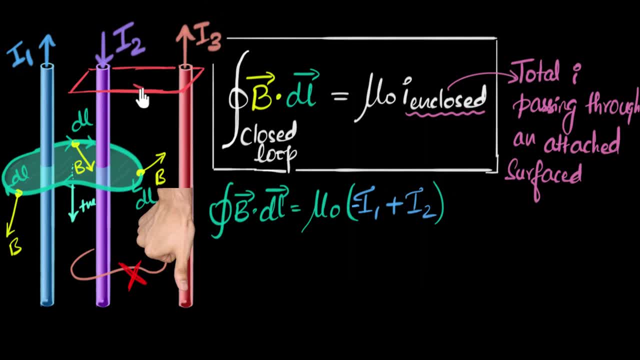 somewhat like this. And this time let's say we walk this way and calculate b dot dl. Can you pause the video and think about what will be the closed loop integral of b dot dl? over here It's gonna be mu naught times something. 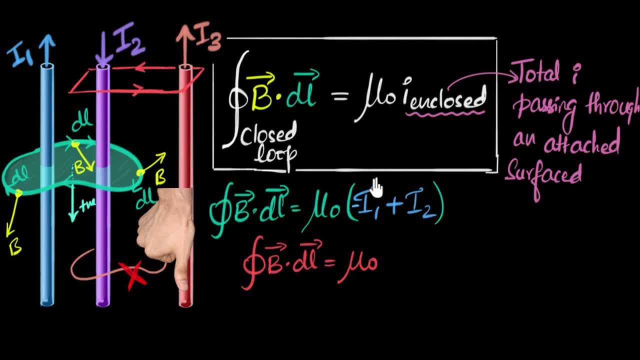 What will that be? Can you pause and think about this? All right, so the first step would be to dip this in a soft solution and attach a flat surface to it, And now the current that penetrates through this surface will be our enclosed surface. 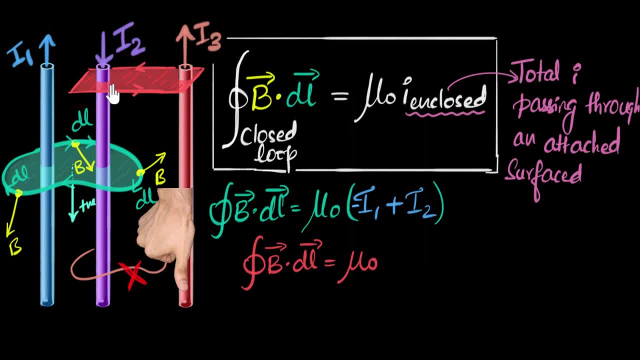 And you may be wondering why should we attach a surface? We'll talk a little bit about that towards the end of the video. But the current that penetrates is I2 and I3. And now we need to know which direction is positive. 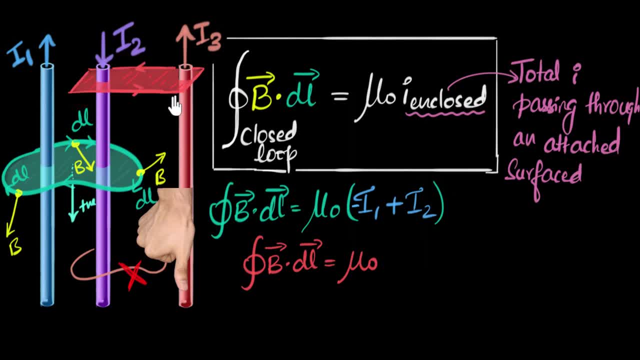 For that we use our right hand thumb rule. In this case, we are moving in this direction And so if I use my right hand now, keep it over here somewhere. Okay, if I move my right hand now, now notice the thumb points upwards. 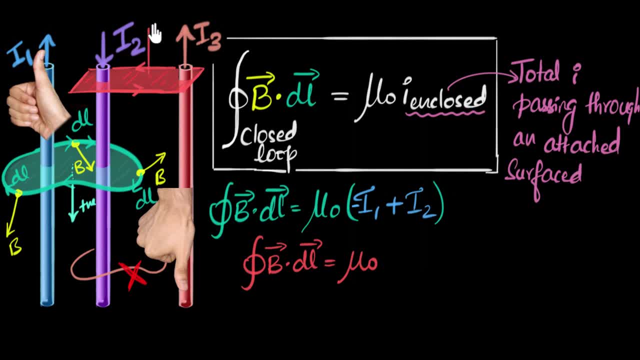 So upwards is my point And I2 is my positive. So this is now positive. So what I end up getting is plus I3.. So I3 becomes my positive current. I2 becomes my negative current, So minus I2.. And I1 is not in the picture. 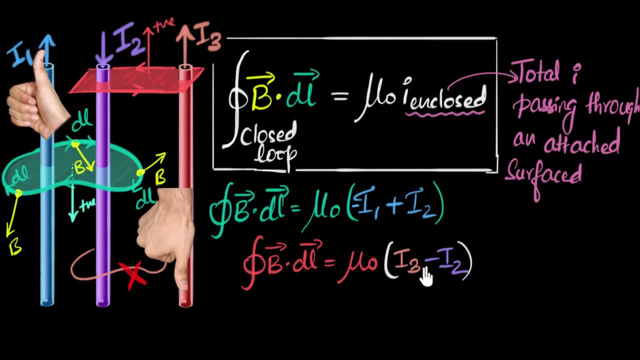 because I1 is not penetrating to that surface. And there you go. This is how we use Ampere's Circular Law, And before we wind up, I want to talk about some important characteristics of this law. First of all, this law can be derived. 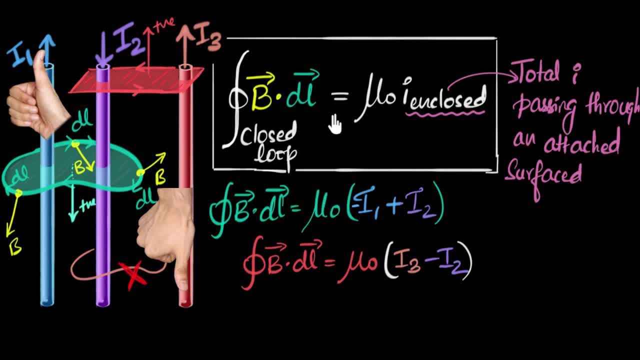 from Biot-Savart Law And you can derive Biot-Savart Law from this law. So they're both equivalent And we use whichever one is more convenient in our given situations, And sometimes when things are very symmetric, we go for Ampere's Circular Law. 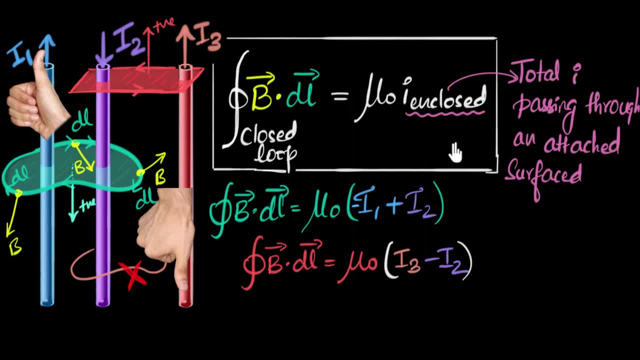 because it makes our calculations simpler Again, something we'll see in future videos. Secondly, on the right hand side, we only consider currents that are enclosed by the loop Right, So for, in this example, only I1 and I2, but not I3.. 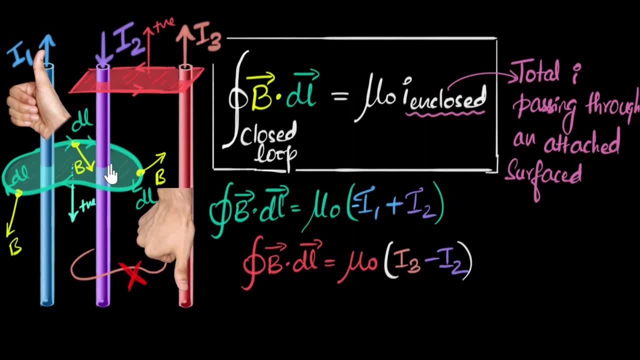 But what about the magnetic field On the left hand side? Is that only due to the enclosed currents? No, That is the total magnetic field. So the magnetic field which we are considering is due to all the currents, enclosed and non-enclosed. 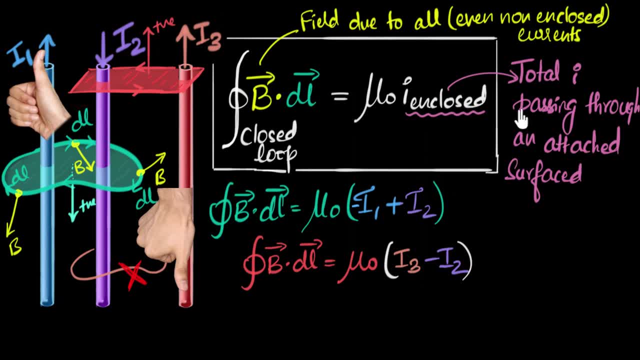 So how does that work? Why is it on one side we have total field, but on the other side only the enclosed one matters? Well, that's because, again, this is like mathematically, we'll not get into the details, but what happens is. what this means is that 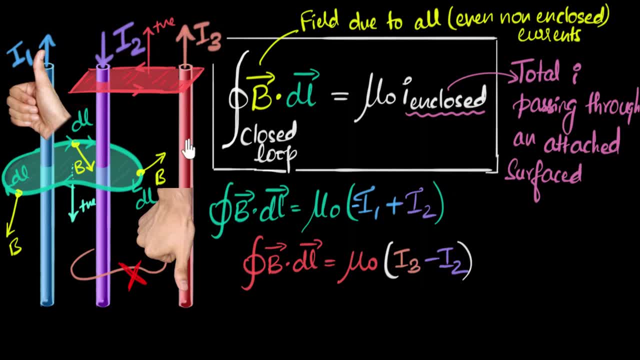 the contribution of BDL provided by the non-enclosed currents. they add up and become zero, So they end up giving zero contribution. So you can imagine, as you walk around this loop, when you, in some cases, the contribution of this is positive. 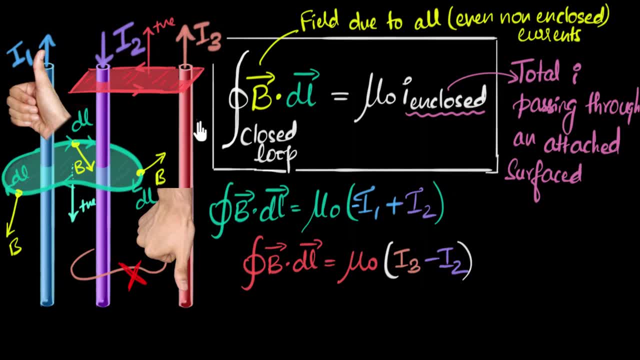 in some places the contribution is negative, and so the total contribution of them is zero. This is very similar to what we saw in Gauss's law: The total electric flux only depends upon the charges that are enclosed by the surface over there Right.